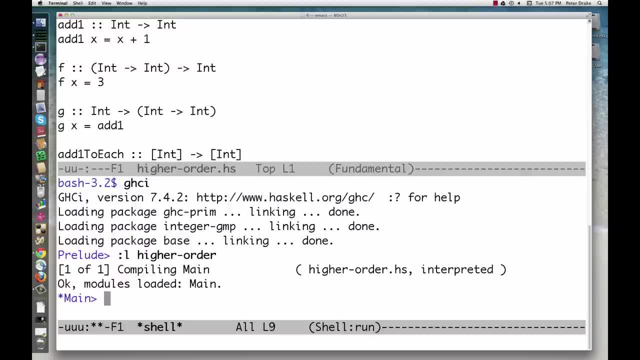 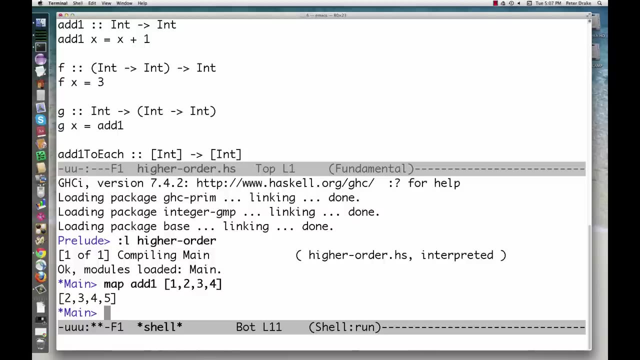 that is, functions that accept or return other functions. A much handier, higher-order function is map. Map takes a function and a list. It returns a list made by applying the function to each element of the old list. We could have defined a function to do this work. Map makes this much easier. 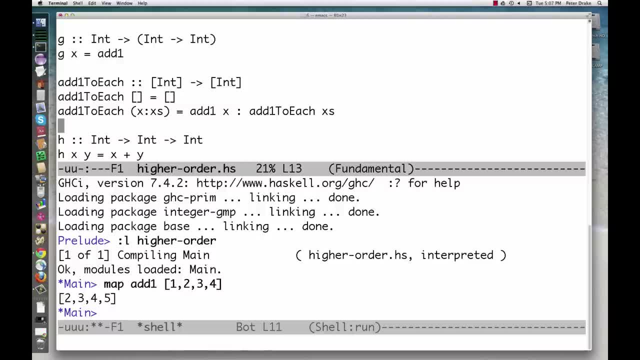 by separating the processing of the list from the processing of the function, The processing of the list from the action being performed on each element By capturing a common pattern of computation map lets us avoid a lot of redundant code. We don't need to define separate functions. 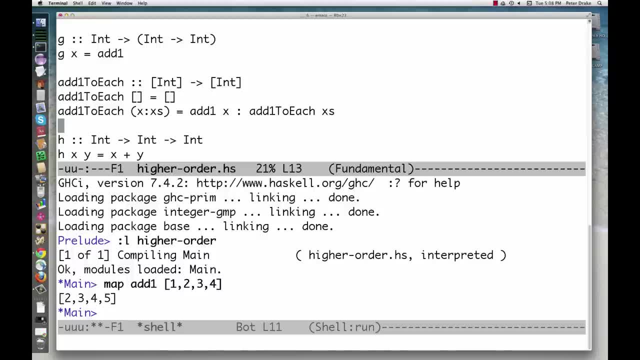 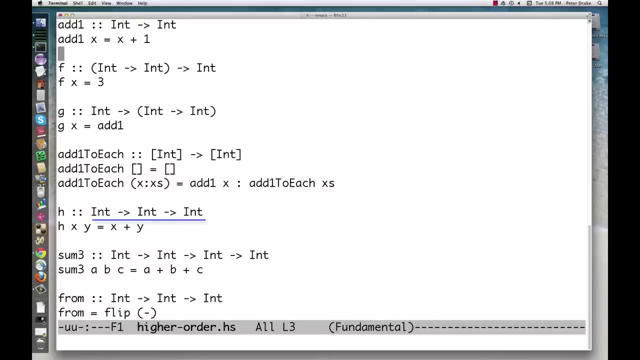 for triple each, square each and so on. Now consider this function. So far, we have imagined that this function takes two ints and returns a third one, but that's not really what's going on. Take a look at the type signature. If the function takes two ints and returns a. 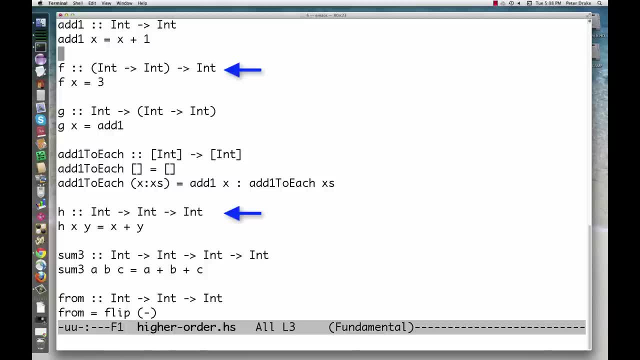 third one. it must be one of the two. If the arrow associates from left to right, then h has the same type as f. If the arrow associates from right to left, then h has the same type as g. It must be one of the two. It turns out that it's the second one. H takes an. 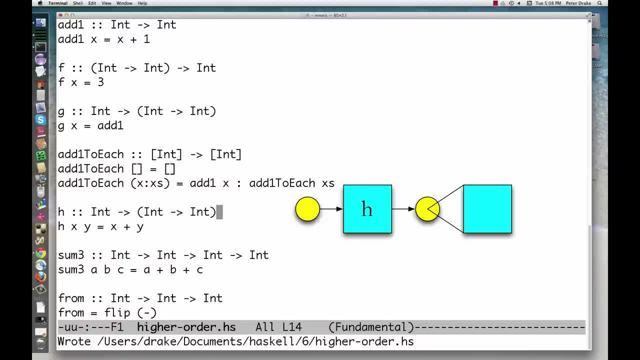 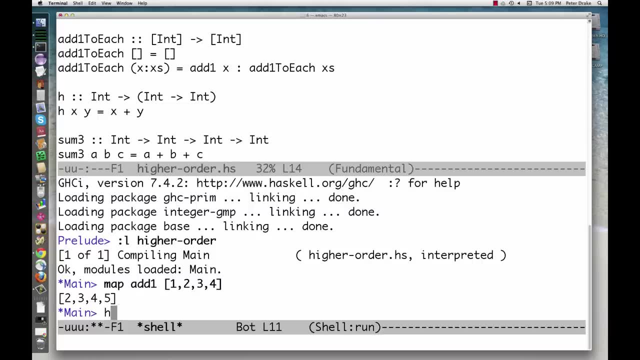 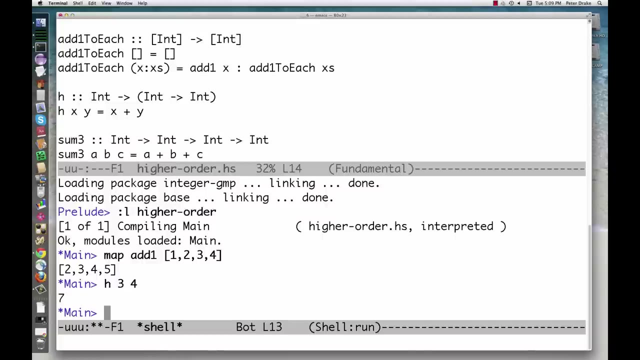 int and returns a function that, in turn, takes an int and returns an int. Now, wait a minute. We know that this function is perfectly happy to take two ints. What's going on Again? think about associativity. This is the same as either h of three of four. 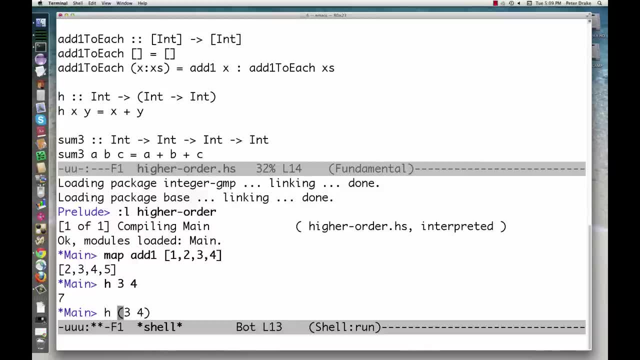 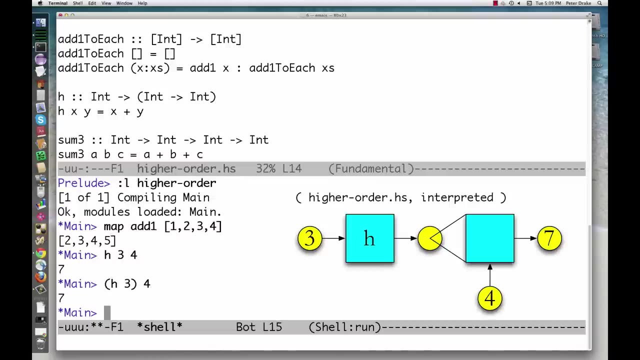 or h of three of four. Asking for three of four in the second case doesn't make any sense, so it must be the first one. We take h of three, which returns a function, and apply it to four. So what function is? 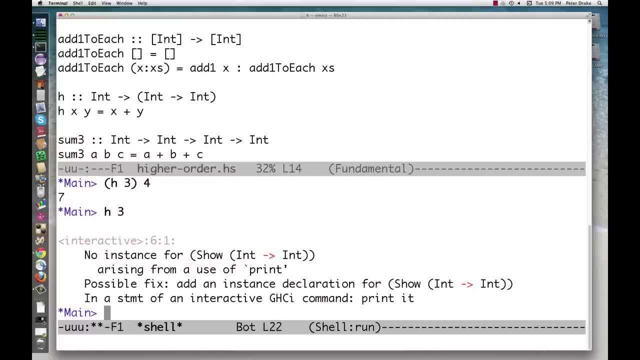 returned. when we ask for h of three, We get an error message, but Haskell is not telling us that taking h of three is illegal. Haskell is just saying that it doesn't know how to print the resulting value, which is a function of type int to int. We can store this value. 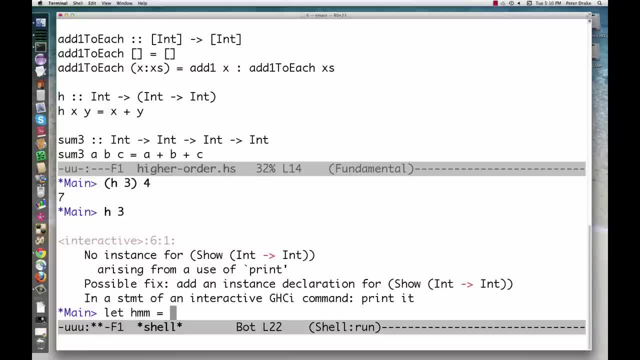 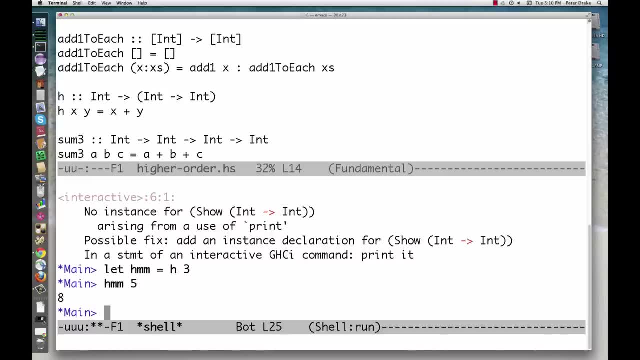 in a variable. Now we have a function that we can apply to a number. The function hmm then adds three to its argument. It is the result of partially applying the function h. Any Haskell function that appears to take multiple arguments can be. 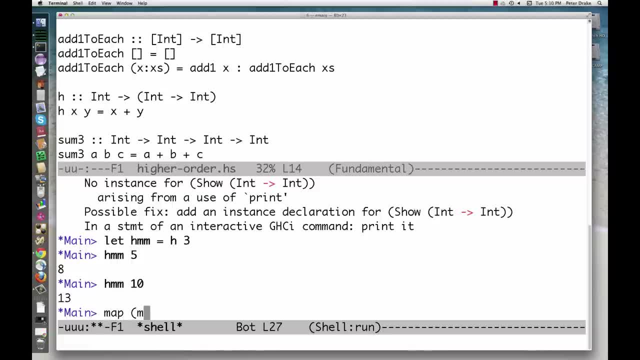 partially applied this way Here. we partially applied max to get a function that returns the max of three and its argument. We then mapped that function, which has no name, over a list. In fact, every Haskell function takes one argument and returns one value. If it appears otherwise, it's because 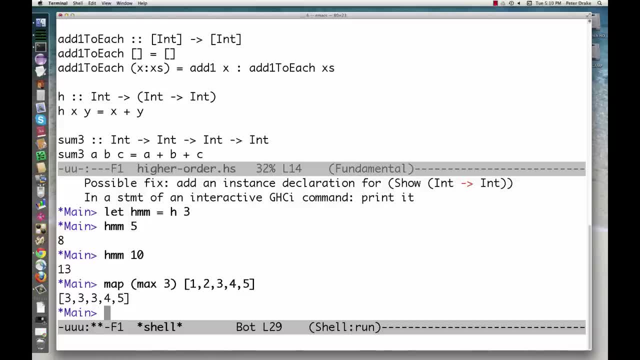 applying the function really involves creating a series of functions and applying each one to the next value. The type here could be written as: Sum three takes an int and returns a function. That function takes an int and returns another function. That function takes an int and returns an int. 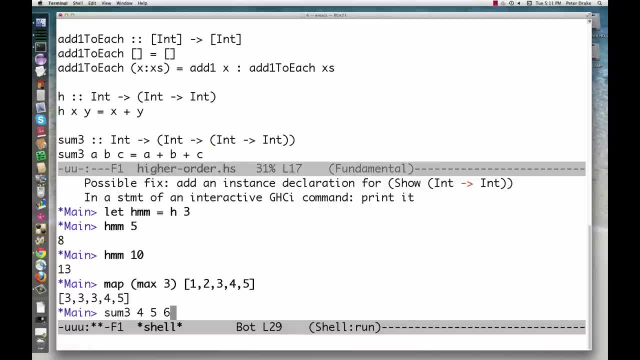 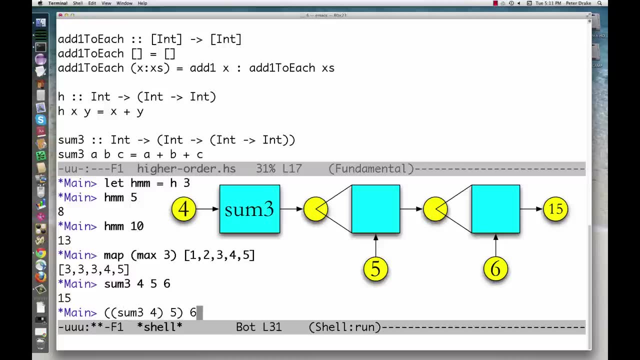 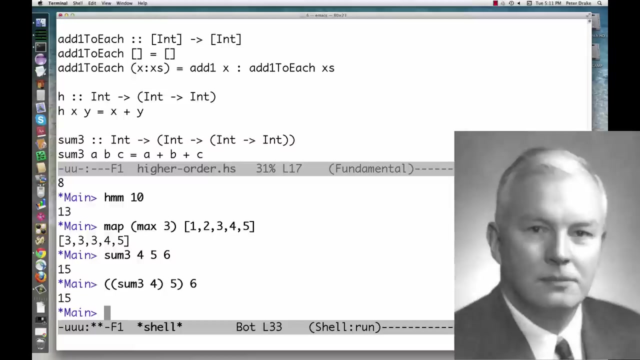 When we ask for, We are really asking for. Haskell allows us to leave out the implied parentheses in both the type signature and the function application. Functions that are broken down like this are said to be curried after Haskell. curry Currying is possible in all functional languages. 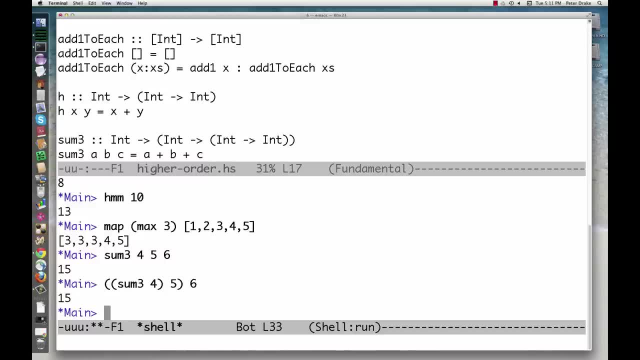 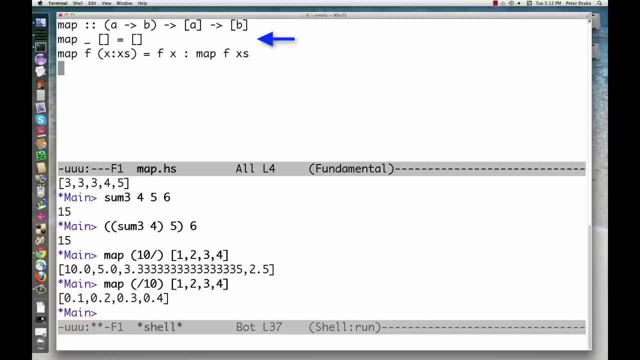 In Haskell all functions are automatically curried. InFix operators are also curried. Conveniently, we can supply either of the two arguments. Map is built in, but it could be defined like this, Strictly speaking, because it is curried, map takes a function from A to B and returns. 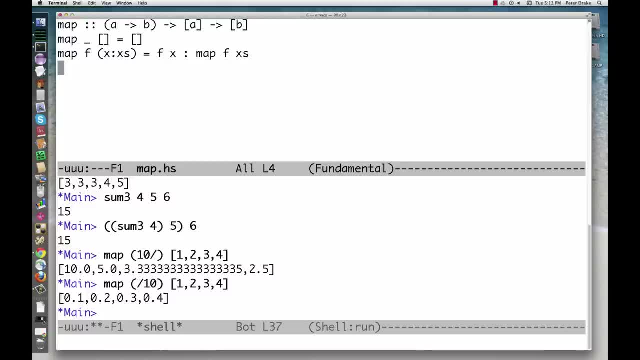 a function from a list of A's to a list of B's. Most of the time, it's easier to imagine that it takes two arguments- a function and a list- and returns a list. We'll often talk about functions as if they take multiple arguments.